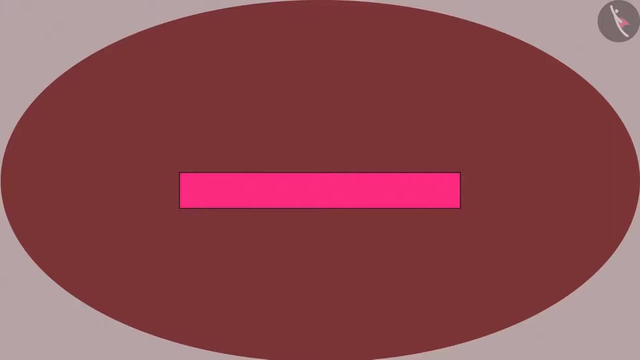 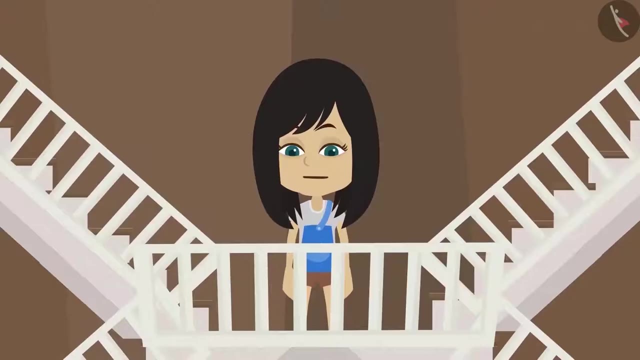 What has he got? This looks like a pink colored box. Look carefully, Neha. this is not a pink colored box, but a yellow colored clock. How can this be a clock? It has no hands at all. This is a pink colored box only. 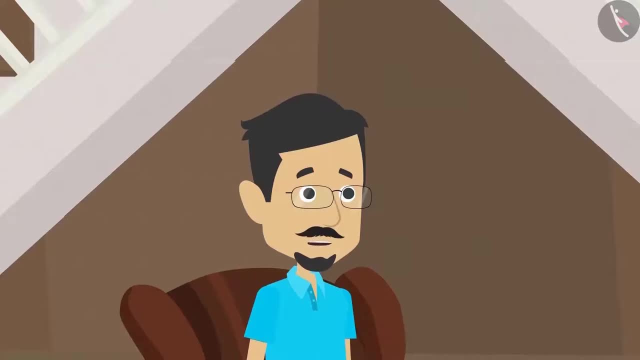 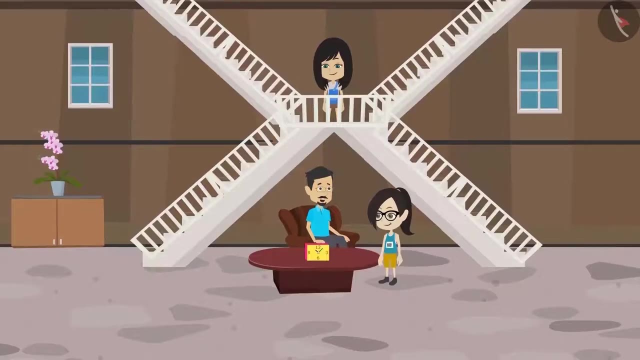 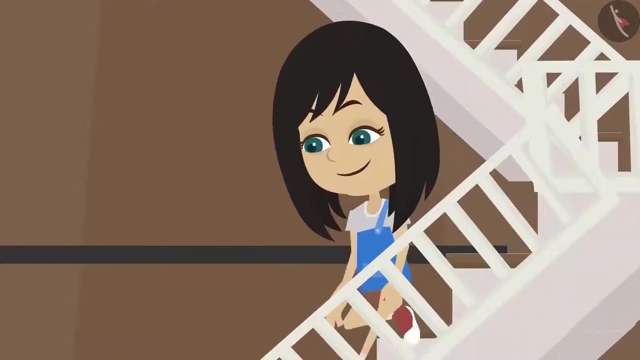 No, Neha, look carefully. Wait, Neha and Vandana. I understand why you are getting confused. I will help you. Vandana, you go to Neha's position and Neha, you come to Vandana's position. Okay, Wow, this clock is very beautiful. 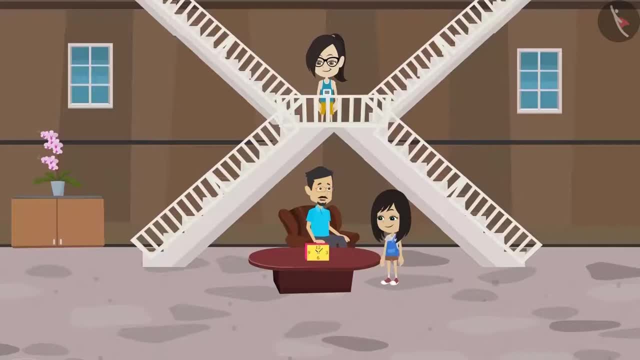 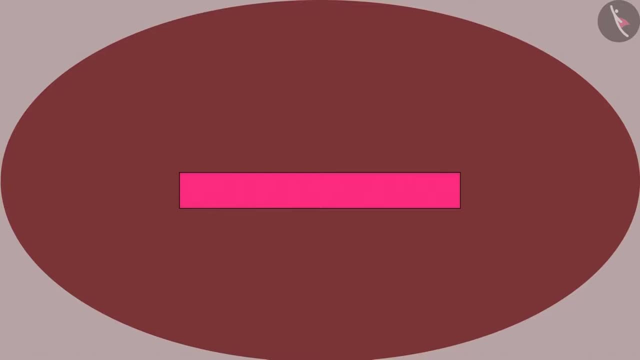 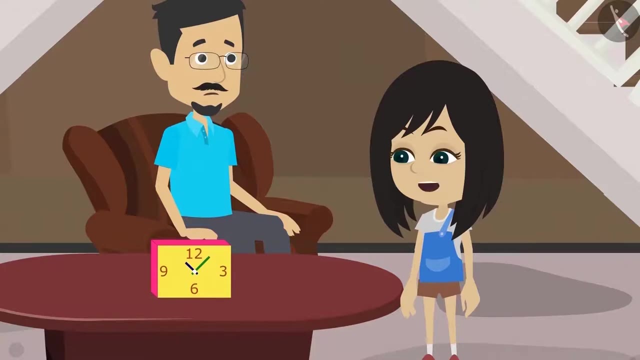 Oh good, you can see the clock now. Vandana, now you tell me how does the clock appear to you? I cannot see the clock. Instead of a clock, I can see a pink colored box. This means the clock appears to you the same way. it appeared to me like a pink colored box. 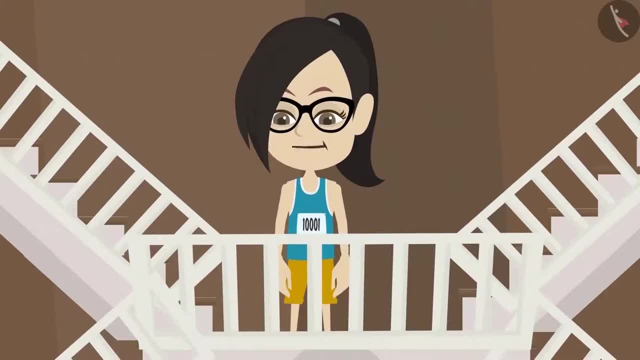 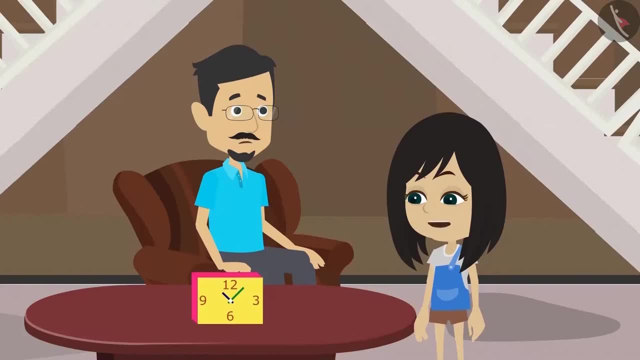 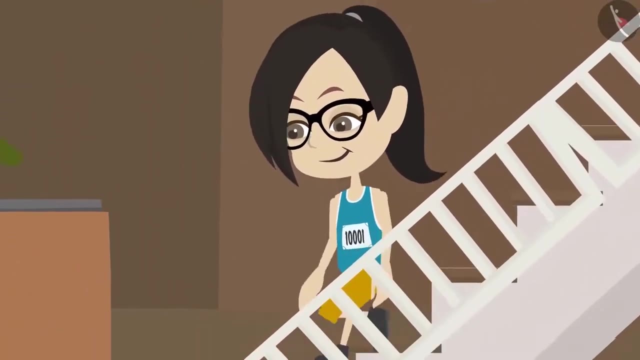 Yes, and you can see the clock, like I was able to see from here. How is this happening, Papa? please explain. Okay, Vandana, you also come here, then I will explain. We live in a 3D world. 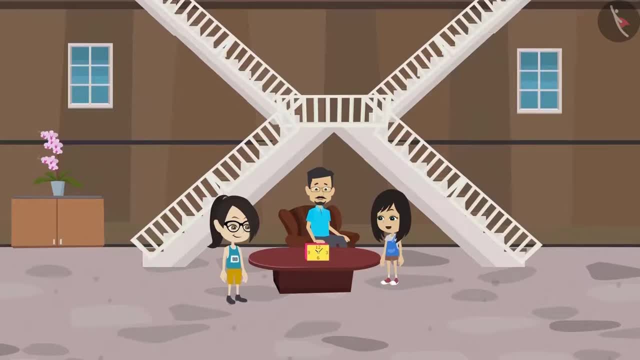 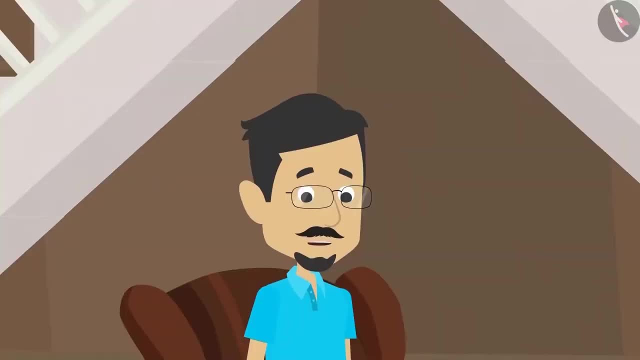 All the objects around us are 3D. What is the meaning of 3D? The meaning of 3D is three dimensional. I am still not clear, uncle. This means that every object has three dimensions. Those are width, height and depth. 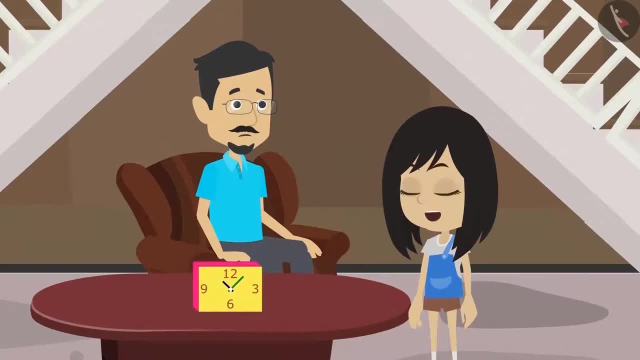 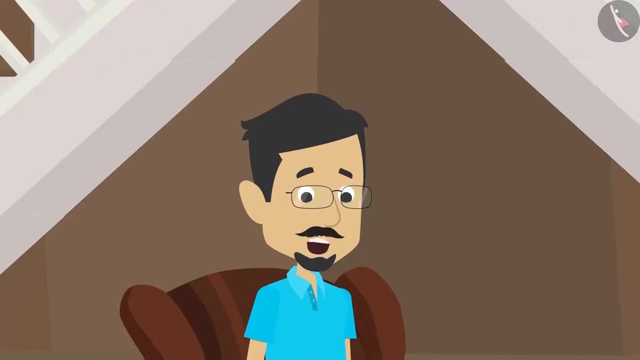 Yes, we had learnt this while learning about bricks: To measure bricks. To measure bricks, We used three dimensions. Yes, and because of these three dimensions, an object appears to be having different shapes when viewed from different sides. For example, when you look from the top, the clock looked like a rectangle. 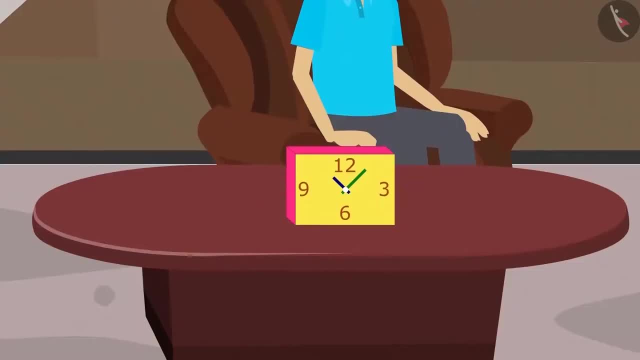 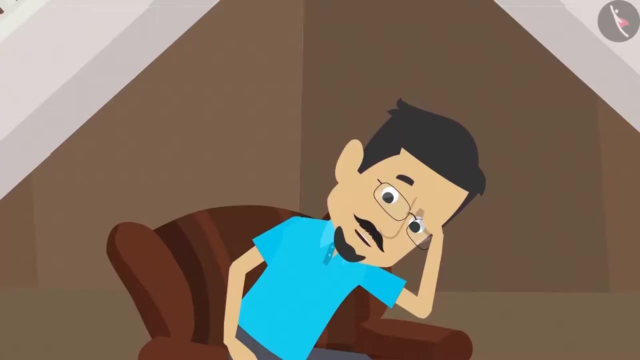 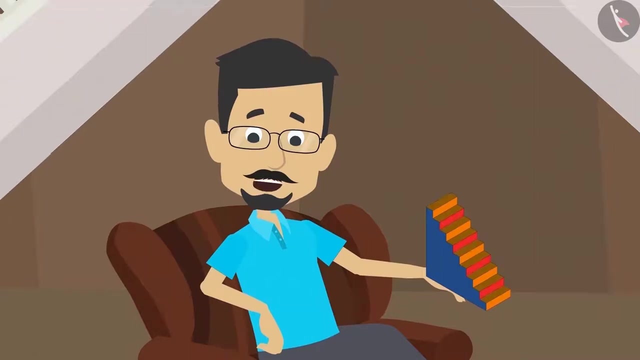 But when you saw from the front, you could see a clock. Now I have understood a little. Let me explain this to you with another example. See, I have a toy That is in the shape of a staircase. I will place this staircase on the table here. 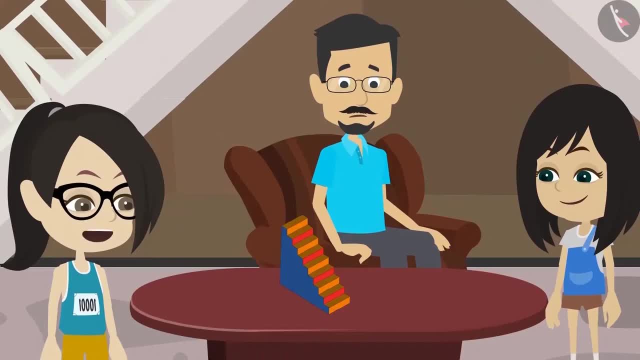 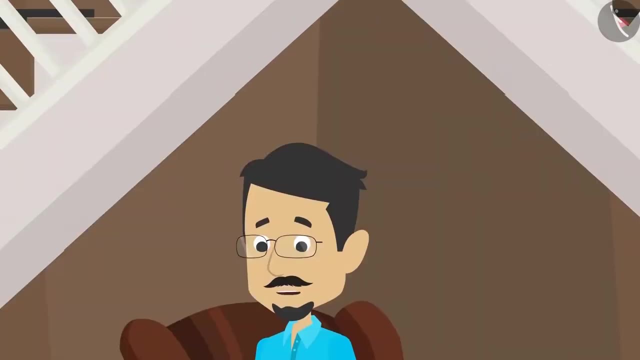 Now we will make a picture of it. That will be fun. Let's start. We will, but wait for a while. We will make this picture from different angles. I will make it from here. I can see this side, Vandana. you make it from here. 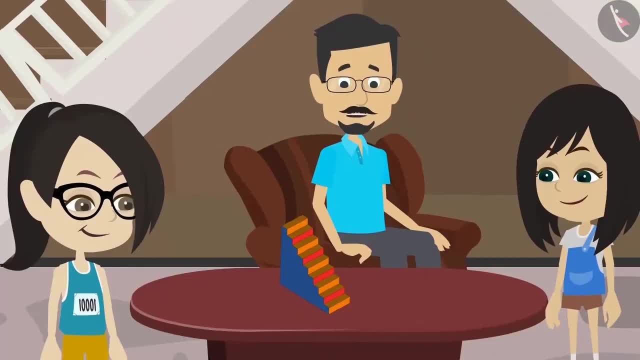 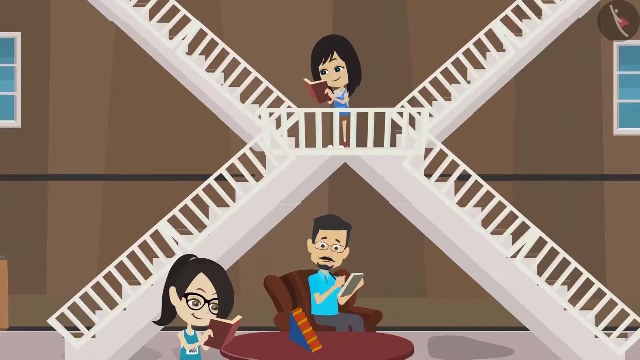 Because you can see it from the front, And, Neha, you make it from upstairs, Because you will then be able to see it from the top. Okay, I have completed the drawing from my side. Even mine is complete. Even I have completed it. 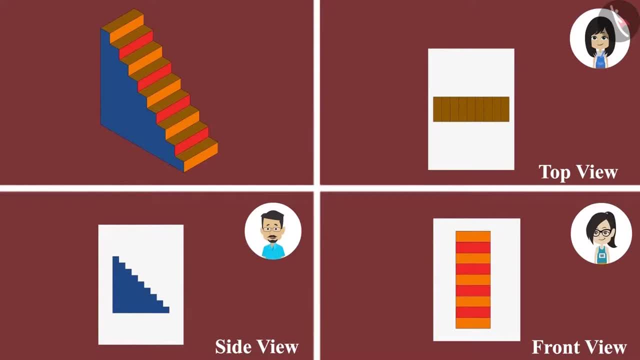 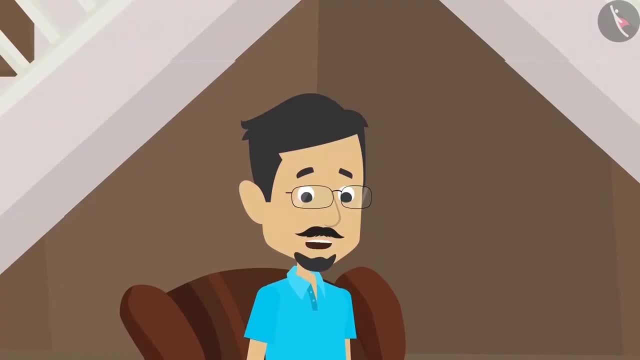 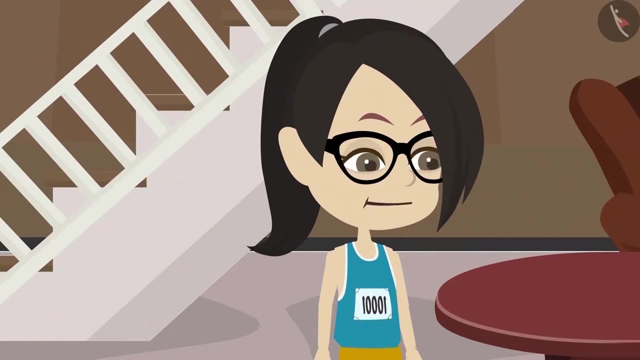 See, the three of us have made a picture of the same staircase, Seeing it from different sides. That's why each of our drawings look different. Now I have understood what is three-dimensional And that when you look at them from different sides, 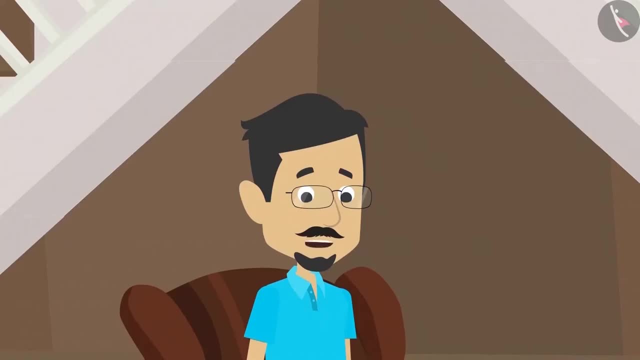 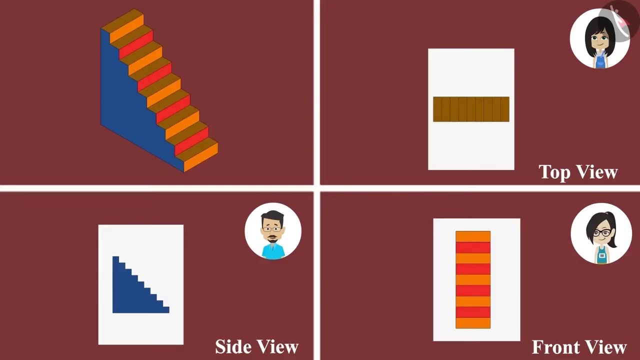 their shapes appear different? Yes, But do you know that to draw the shape of 3D or three-dimensional objects accurately, the drawing is made from three different sides, Like the way we drew this staircase. But what is this three-sided drawing called? 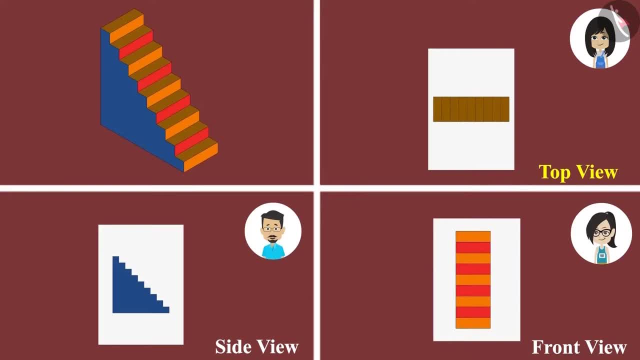 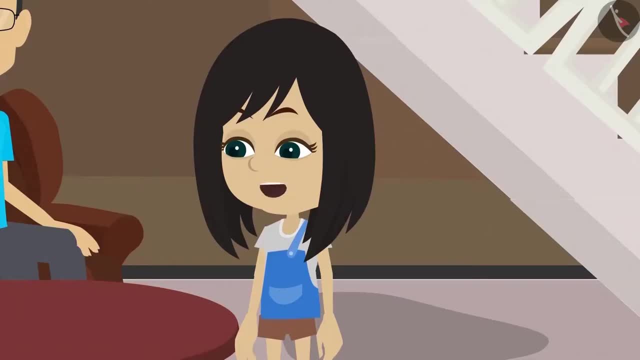 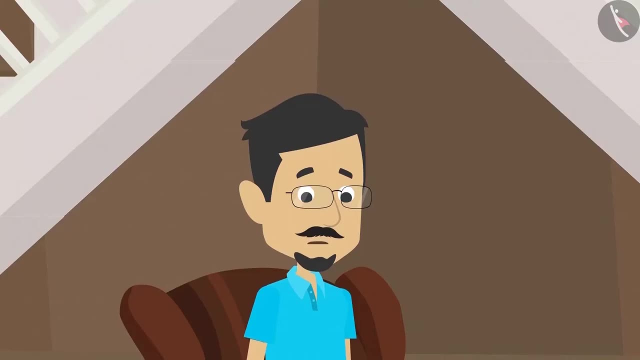 One is called the top view, which tells us how an object will look if seen from the top. This means my drawing is a top view of the staircase, which is a brown-colored rectangle right. Yes, Neha, In addition to the top view, there is another view. 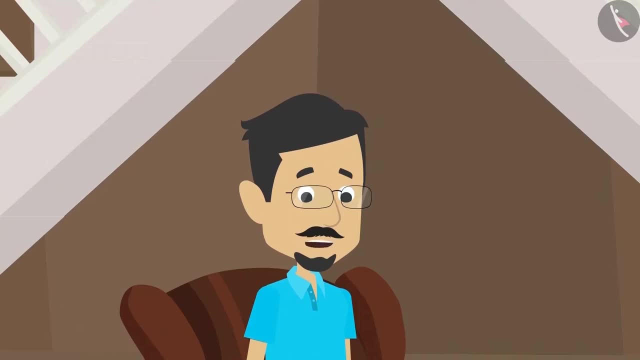 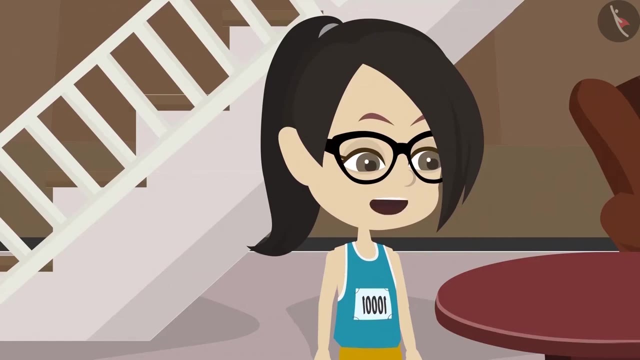 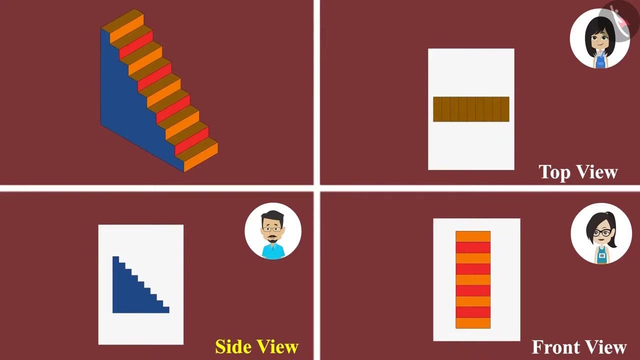 which is called the side view, In that the object is drawn by looking at it from the right side. So does this mean that the drawing you have made is a side view of the staircase, as you meet the staircase, seeing it from the right side of it? 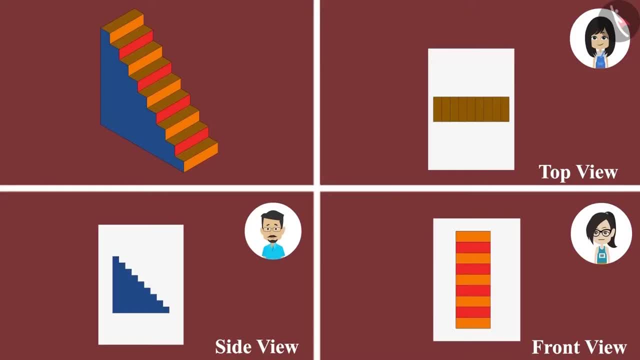 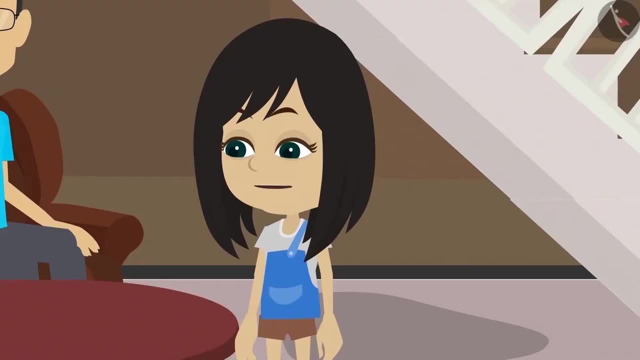 Yes, you are right, Vandana. I drew the staircase from the front, Uncle. which view would it be called? Vandana, this will be called the front view. That means when an object is seen from the front, then its front view will be visible.